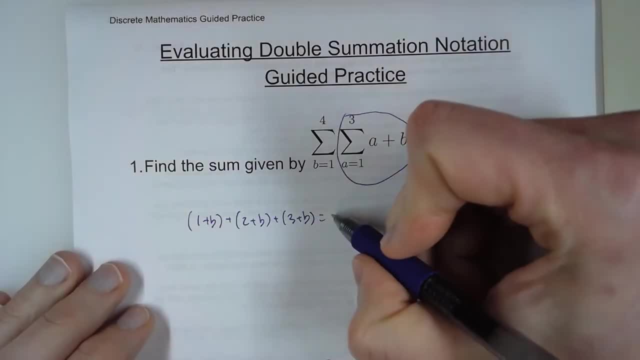 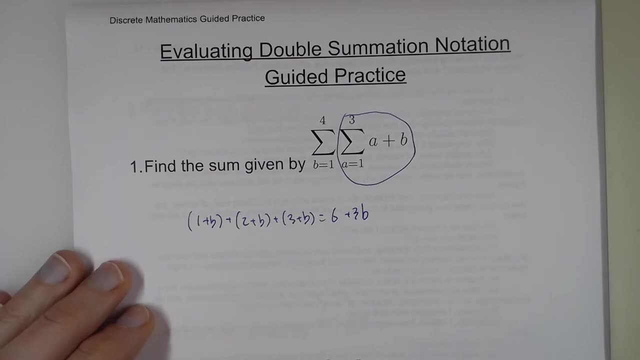 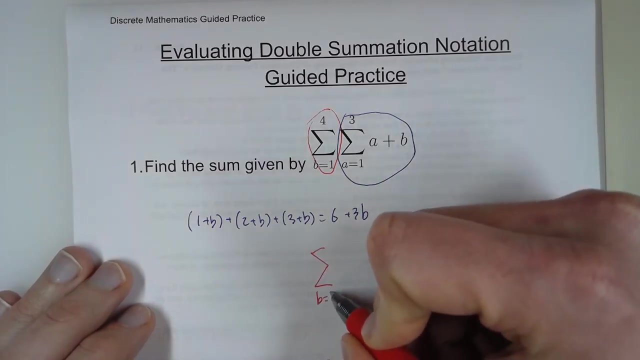 So if I combine all these like terms, 1 plus 2 plus 3 is 6, and b plus b plus b is 3b, But now we still have this outside sigma, So b equals 1 to 4.. So 6 plus 3b. 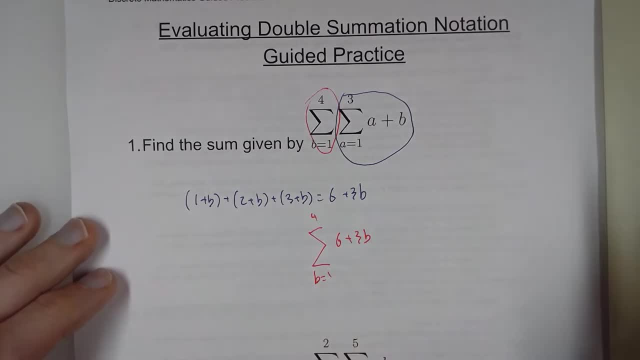 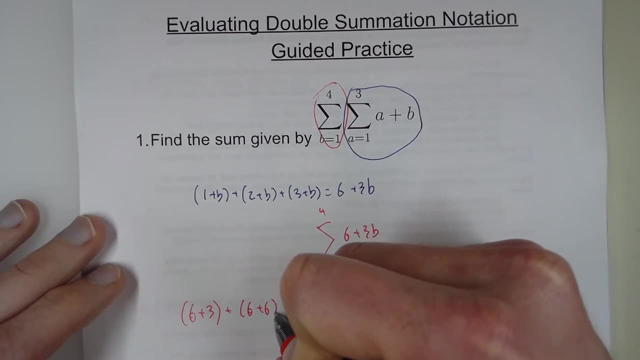 So now we're going to plug in 1,, 2,, 3, and 4-infor-b, So 6 plus 3,, 6 plus 3b, 6 plus 6,, 6 plus 9, and 6 plus 12.. 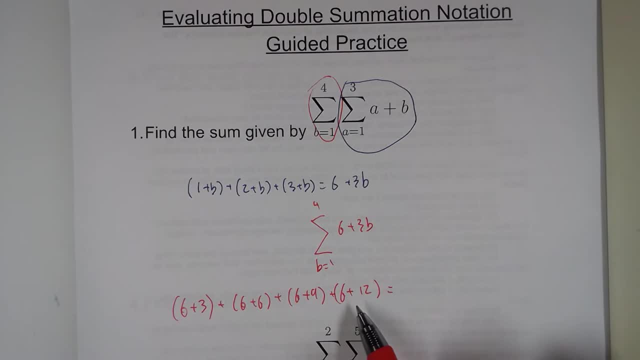 And so 6 plus 6 plus 6 plus 6 is 24.. 3 and 12 is 15.. 6 and 9 is 15.. So if I add that we get 30 plus the 24, gives us 54.. 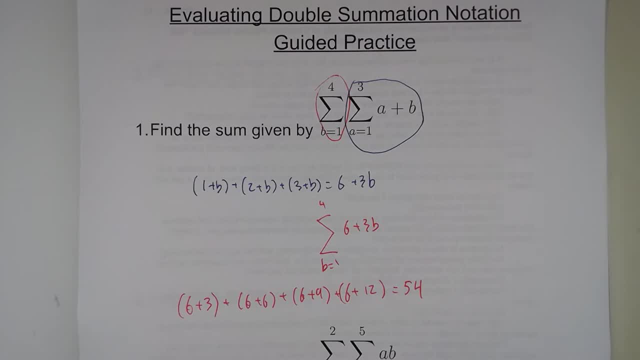 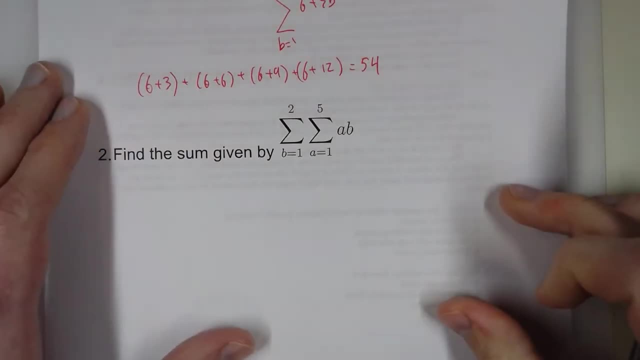 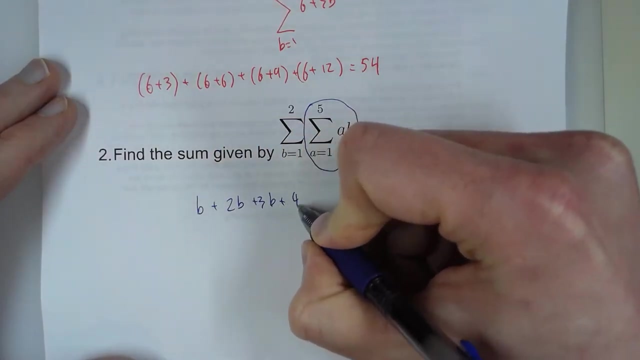 And so that is what this double sum means. So we're going to plug in 1,, 2,, 3,, 4, and 5-infor-a, So that's going to be b plus 2b plus 3b plus 4b plus 5b. 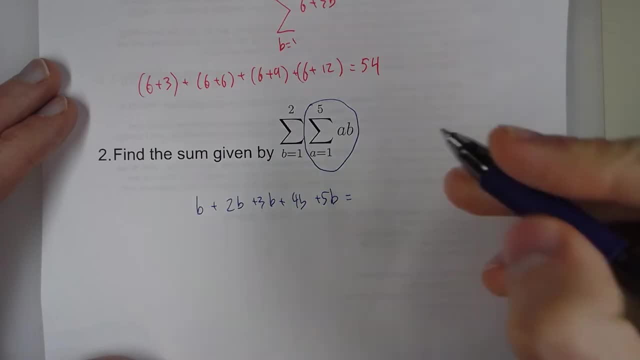 So 1 plus 2 is 3 plus 3 is 6 plus 4 is 10 plus 5.. So that's going to be b plus 2b plus 3b plus 4b plus 5b. b is 15b, is what that equals. 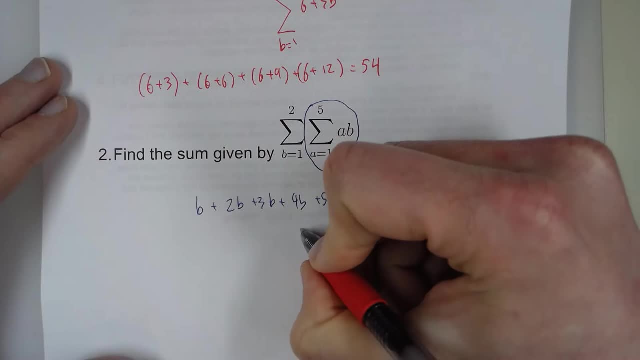 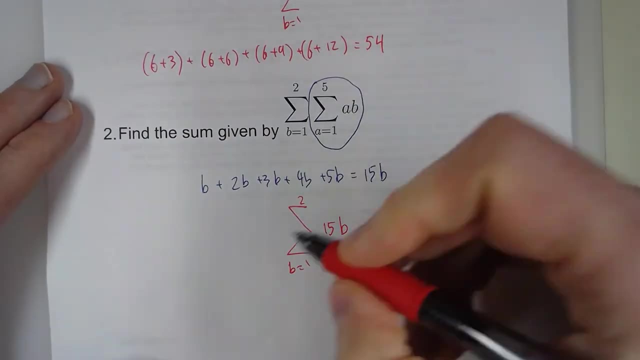 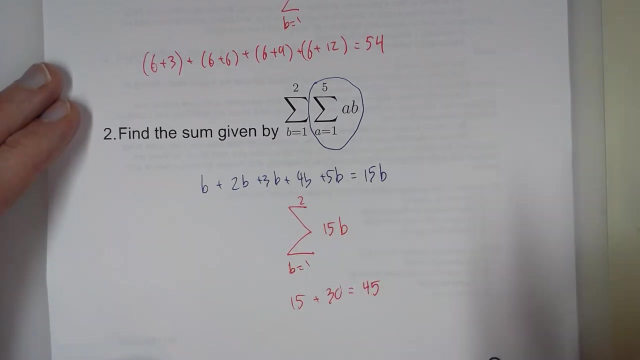 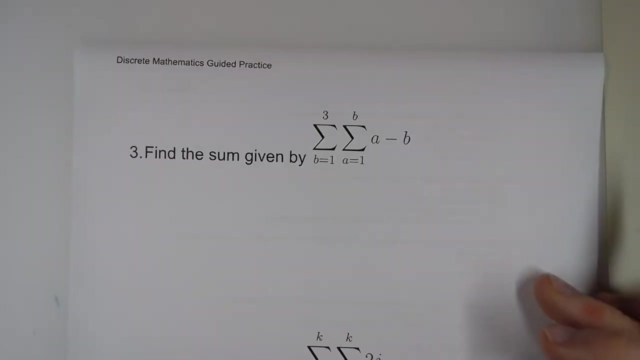 And then we have the other sum. So b equals 1 to 2 of 15b. So we have 15 plus 15 times 2 is 30, which gives us 45 for our sum. Now over here for number 3.. Here this is a little different, because the first one goes from a to b. 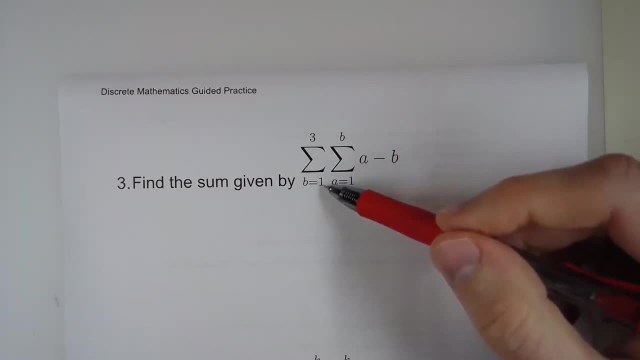 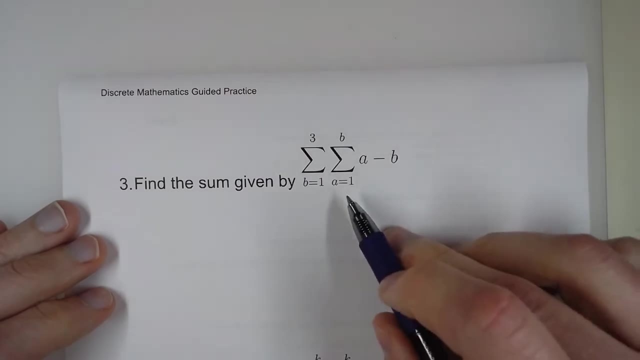 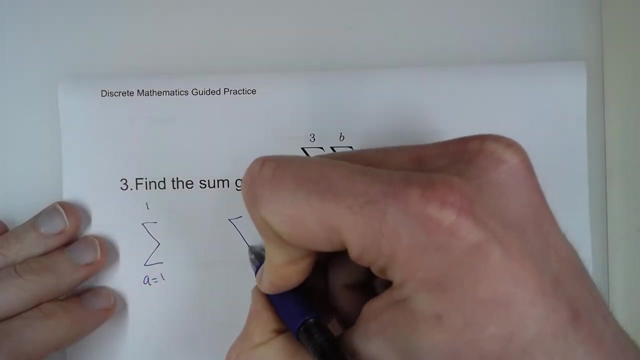 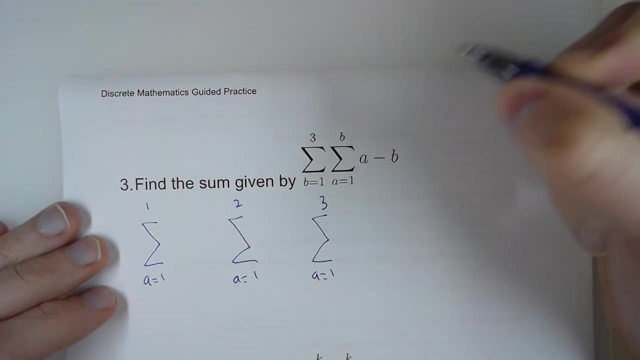 and then this says b goes from 1 to 3.. So what we're going to do for this one is a little different. For this one, we're going to write this as three different sums: a equals 1 to 1, a equals 1 to 2, and a equals 1 to 3.. 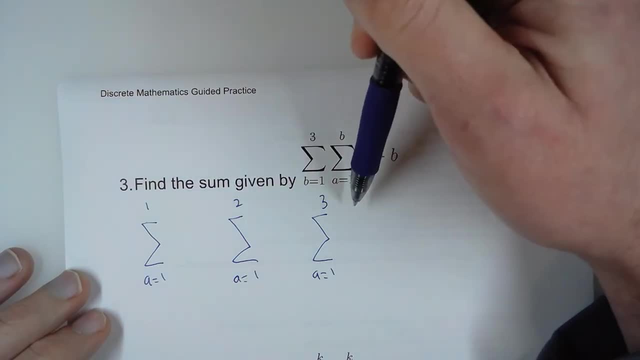 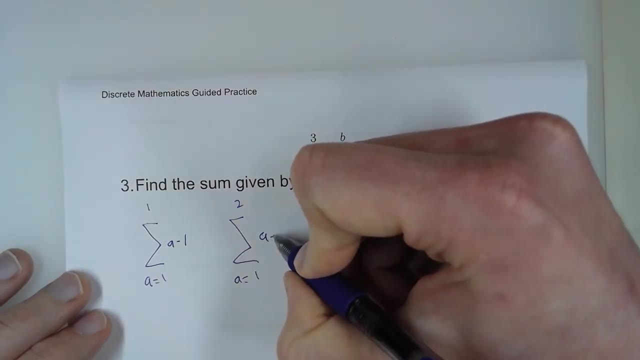 So what I've done is I've plugged 1 in for b, 2 in for b and 3 in for b. So this one is going to be a minus 1, because that's what I said: b equal to here, a minus 2 here and then a minus 3.. 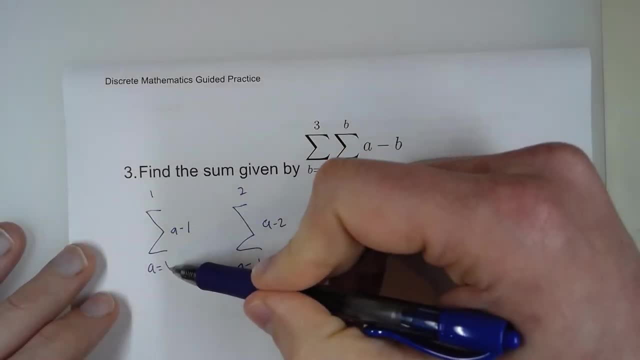 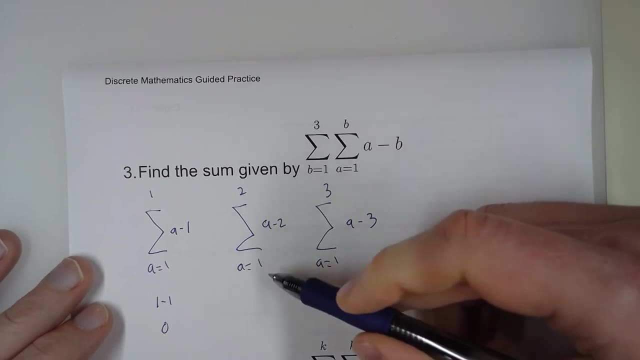 So here I'm plugging in 1 as my first number, but it's also my last number, So this is just going to be 1 minus 1, which is 0.. Here I'm plugging in 1 and 2.. 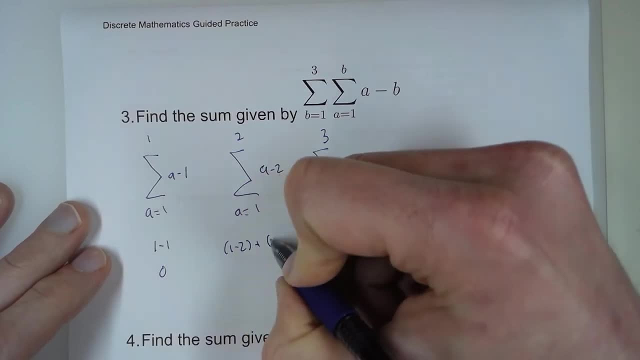 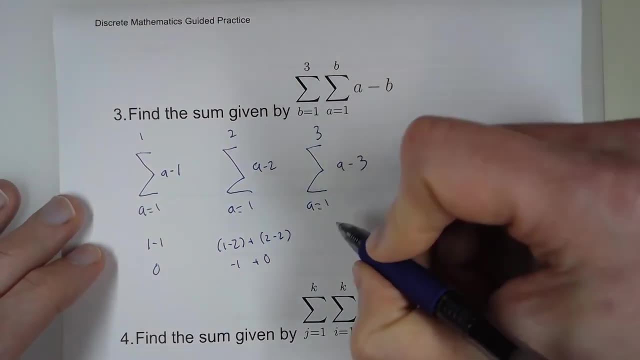 So I have 1 minus 2 plus 2 minus 2.. So I have negative 1 plus 0.. And then here I'm plugging in 1,, 2, and 3.. So 1 minus 3,, 2 minus 3.. 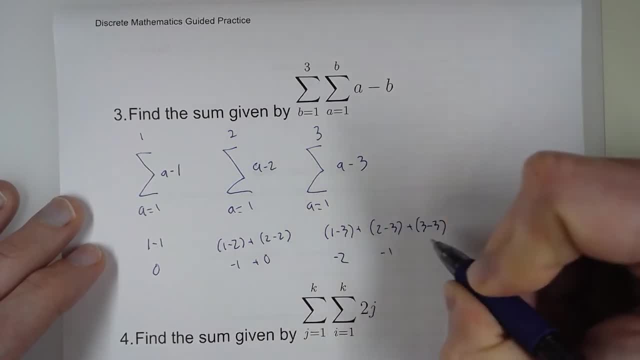 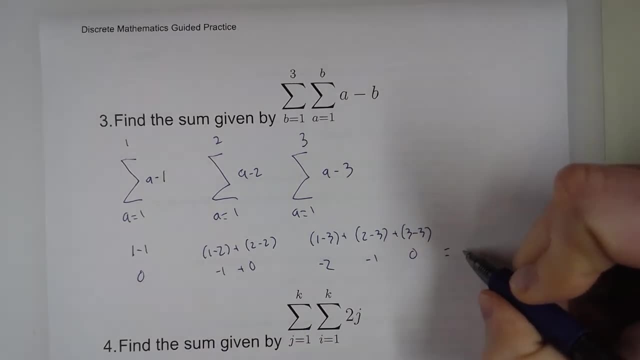 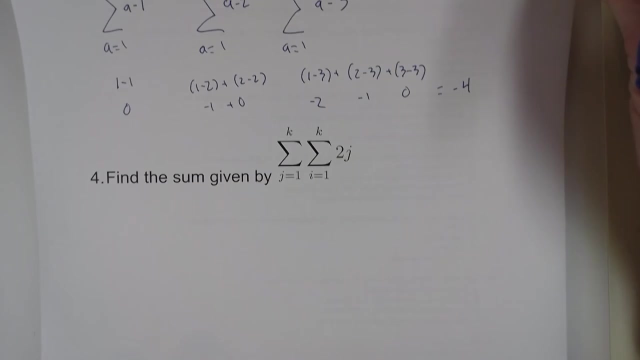 And 3 minus 3.. So negative 2, negative 1, and 0. So when I combine all of those I get a total of negative 4.. And then the last one here. both of these sums add up to k. 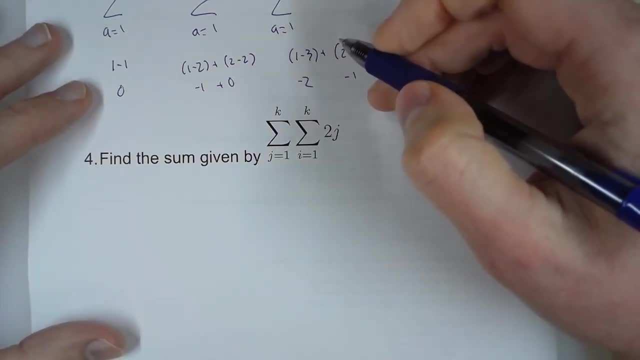 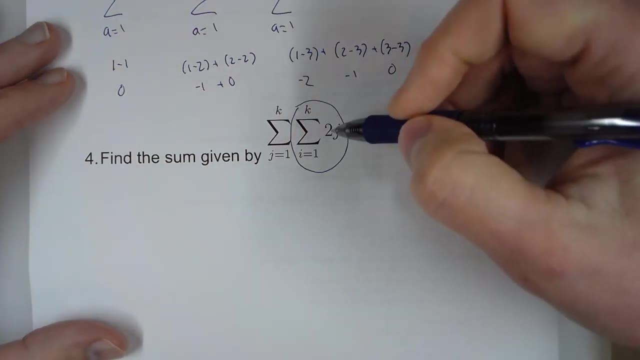 which is neither of the variables. Now here, I'm going to do this like we did numbers 1 and 2.. First I'm going to work on this one, So I'm going to plug in 1 in for i, but there is no i. 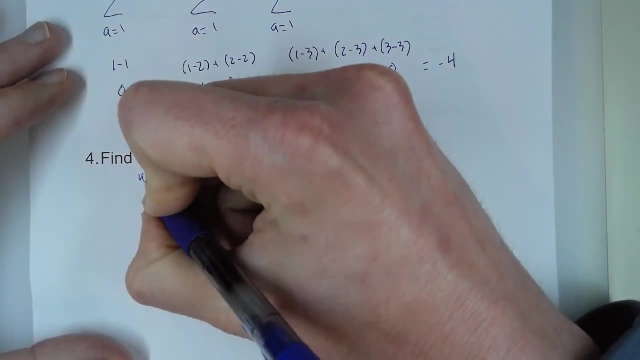 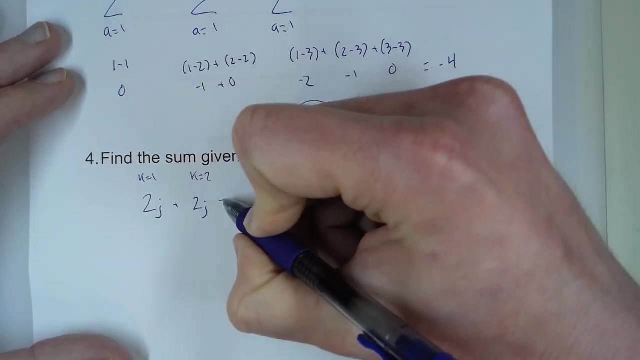 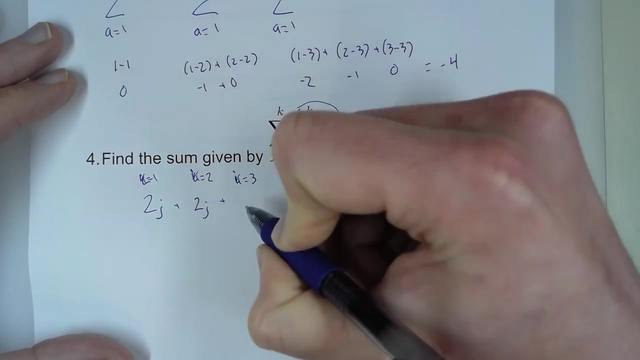 So that means it's just 2j when k equals 1.. And then when k equals 2,, I also get 2j, And then when k equals 3, or, sorry, when i, I get 2j. Now this is going to keep happening until we plug in 2j. 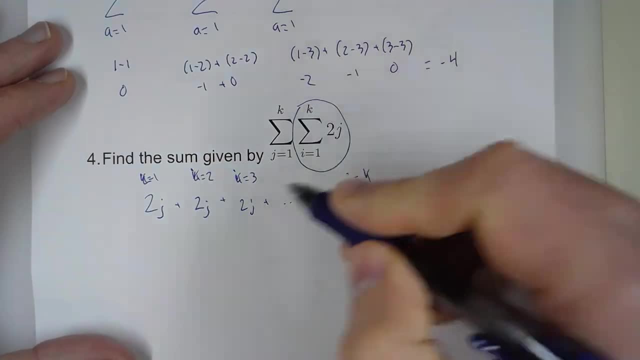 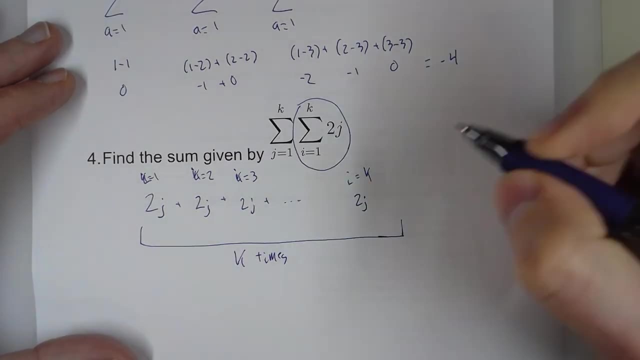 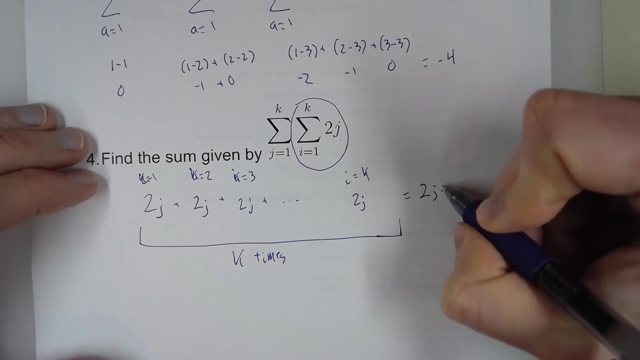 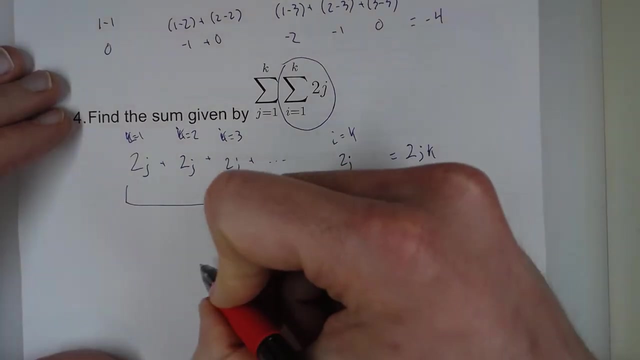